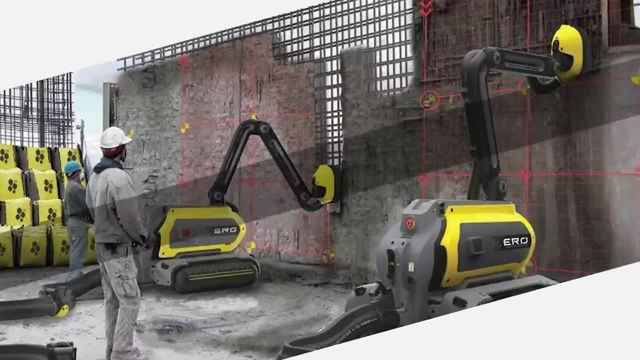 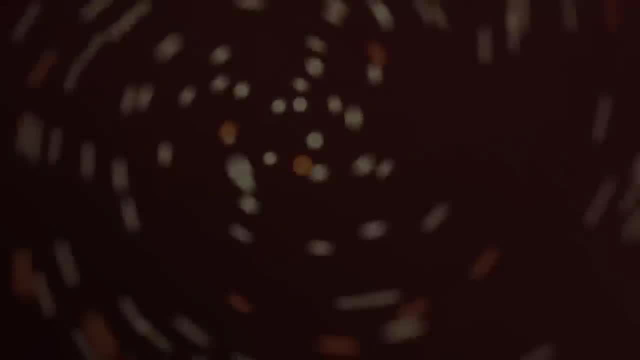 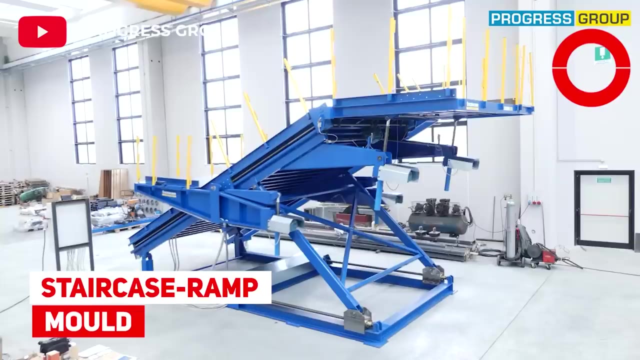 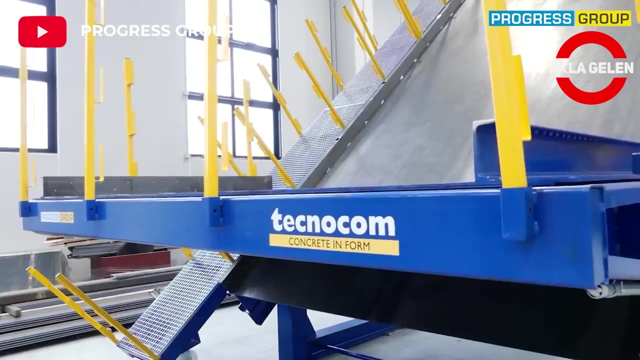 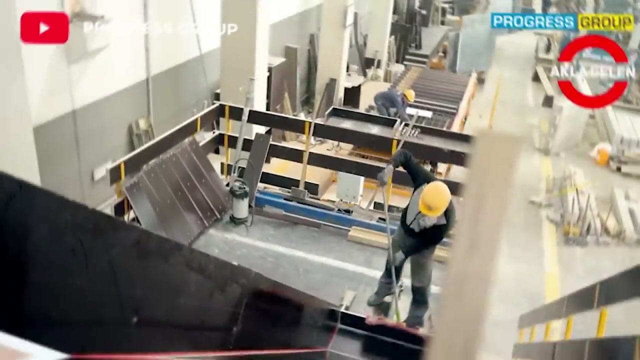 electrical tools or heavy equipment. things would be very difficult. Don't forget to subscribe to the channel and like the video. Let's watch our video now. Staircase Ramp Mold- Automatically adjustable staircase ramp mold with landing. This system is used to make ready mixed concrete stairs using formwork. 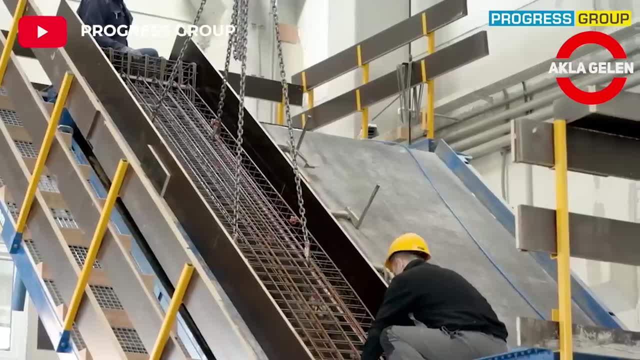 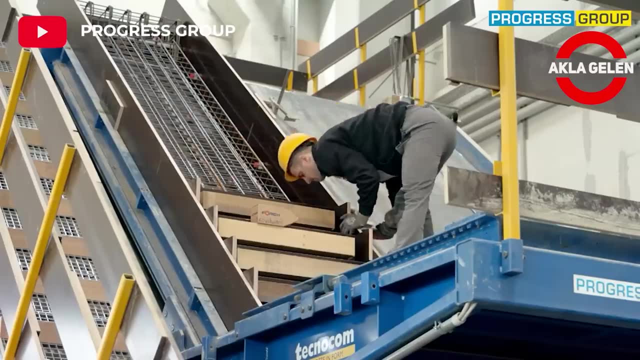 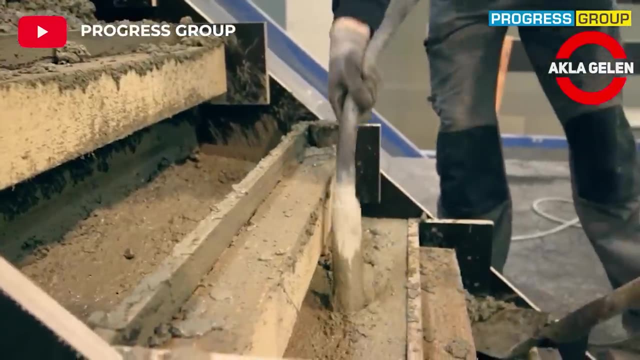 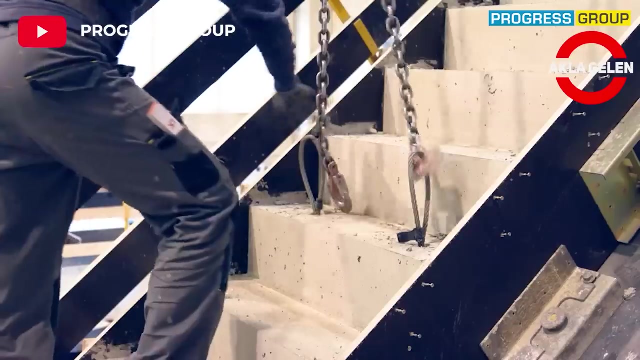 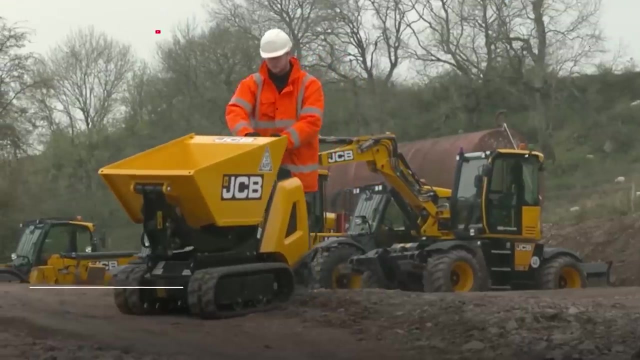 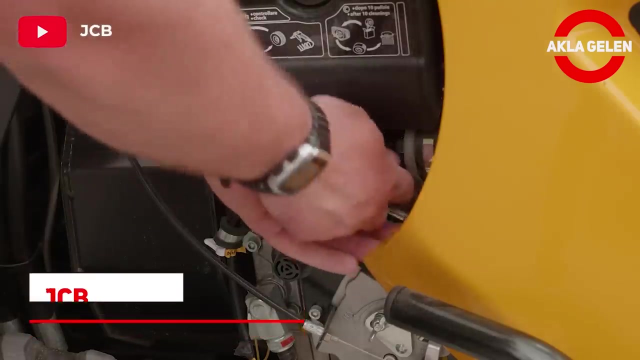 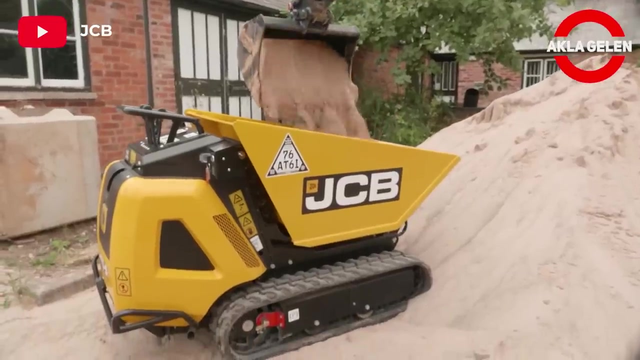 After the iron skeleton is put into the mold, the concrete is poured and the ladder is ready after it dries. High tip dumpster- A compact walk-behind high tip diesel powered mini-dumper. the machine has been designed to save time, energy and money. 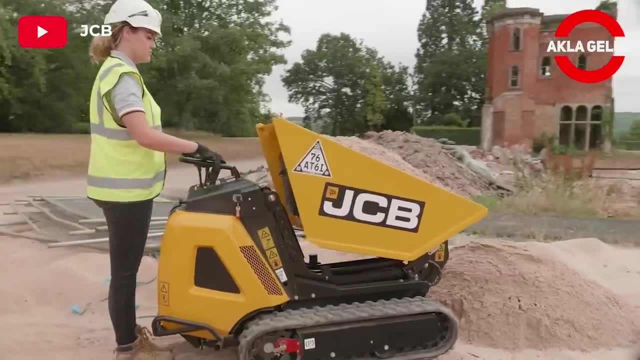 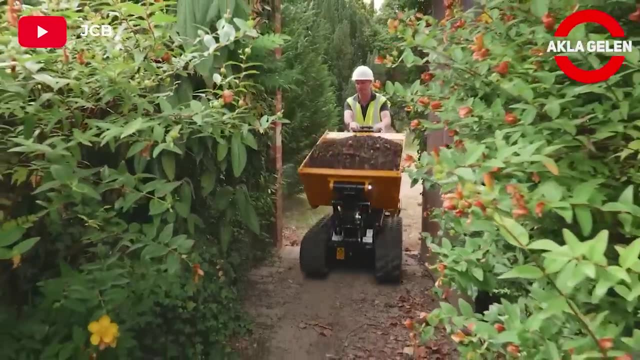 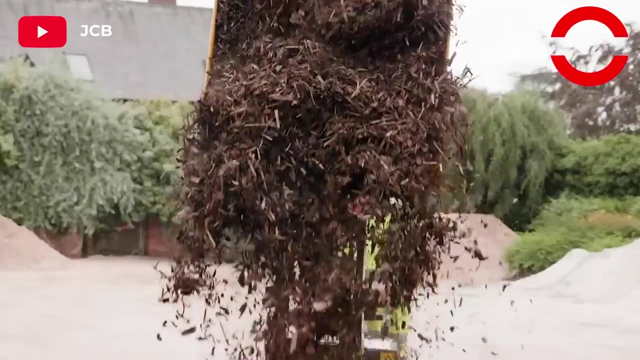 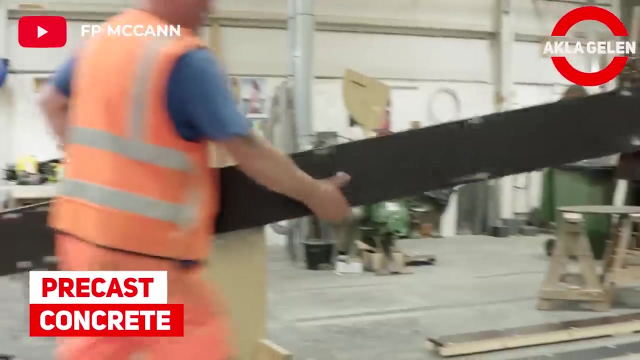 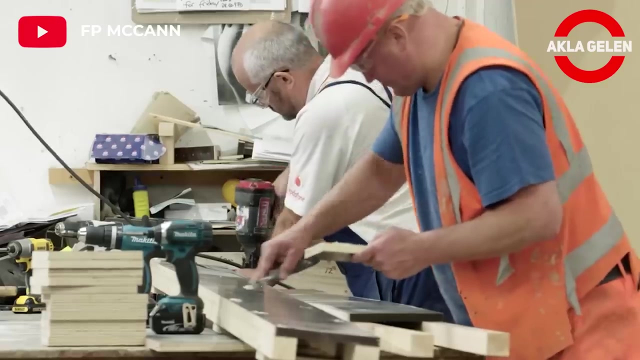 We can call this machine the technological state of wheelbarrows. It is very easy to know that the energy average will be higher than the first week of warranty because they are laserization, useful and modern Precast Concrete. I guess this is one of the easiest ways to build a building. 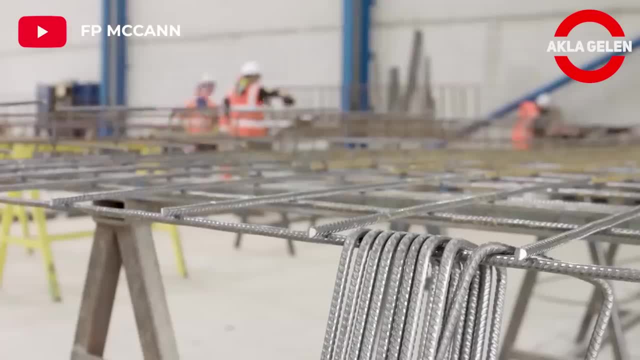 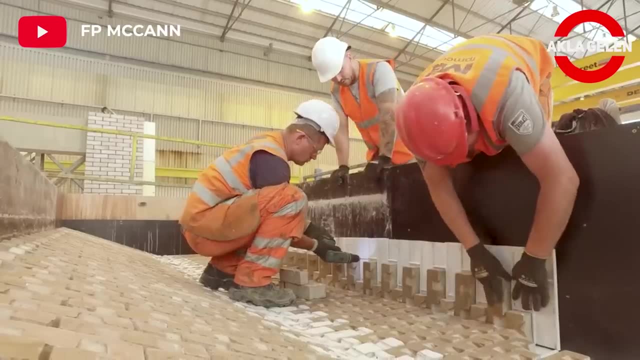 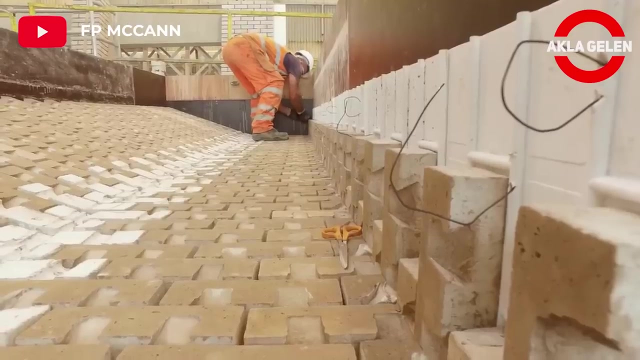 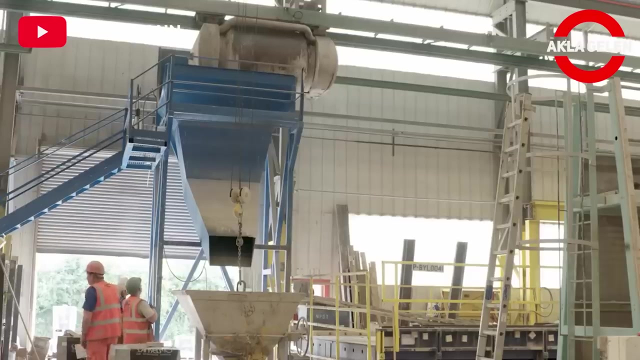 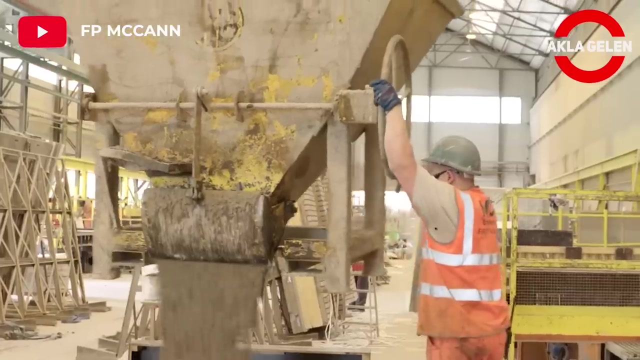 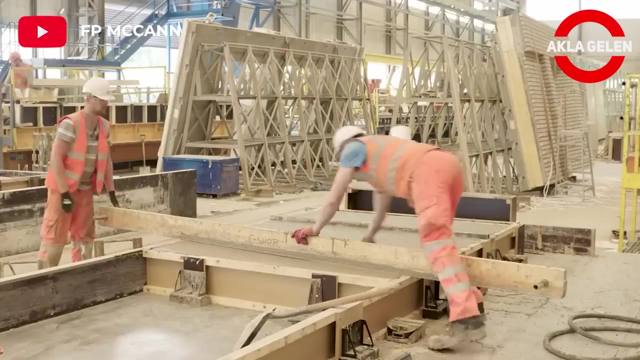 In this system, the walls of the building etc. are manufactured in the factory and only assembled at the construction site. To build a building, the first step must be to build the Citizenship on the ground. The first step is to build the city on the ground. 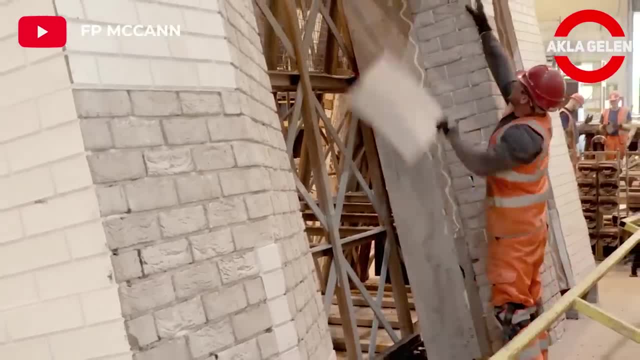 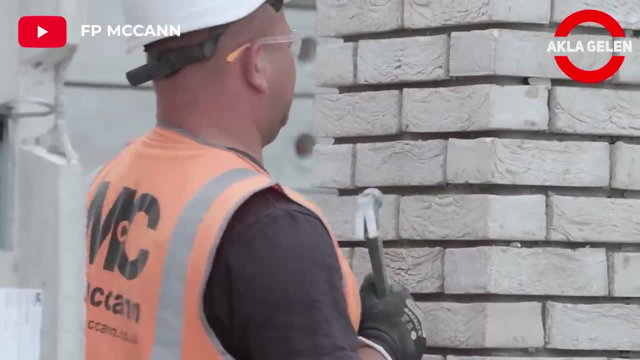 The city must be constructed according to the industrial rules and rules of the city. When the city is built, the building must create the same structure as the city. For example, building a building on the ground with the resistance of the fortress is the first step. The second step is to renovate the building. In this way, the building will house the building. To build a building on the ground, you need to find a structure that mixes by and with the entire structure. This is the start of the first step. 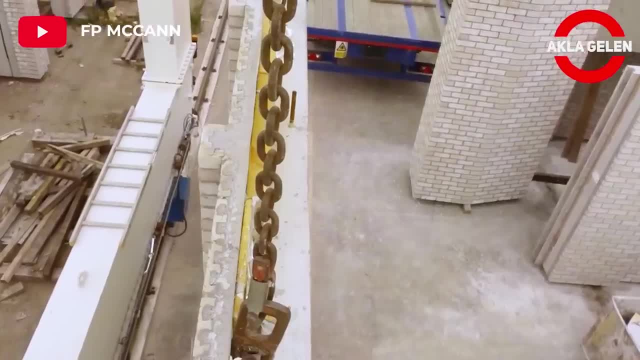 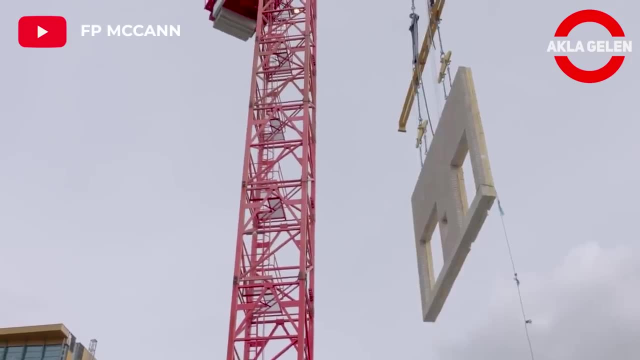 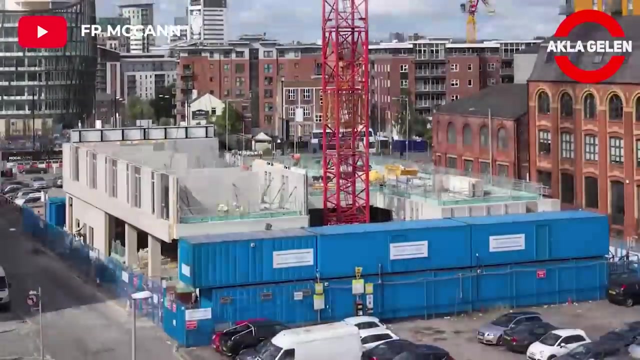 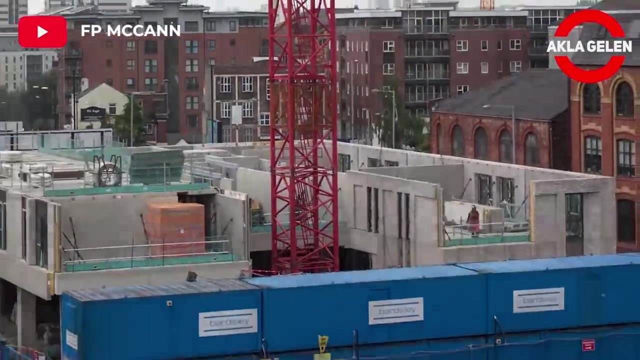 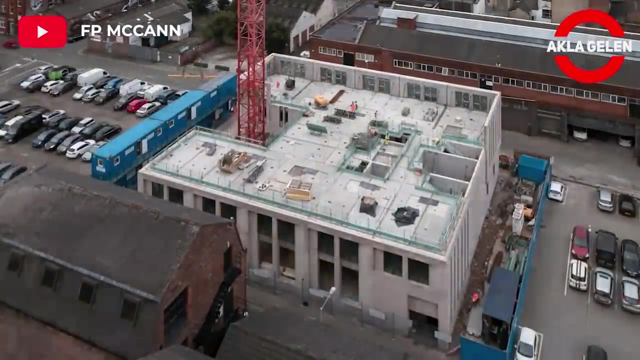 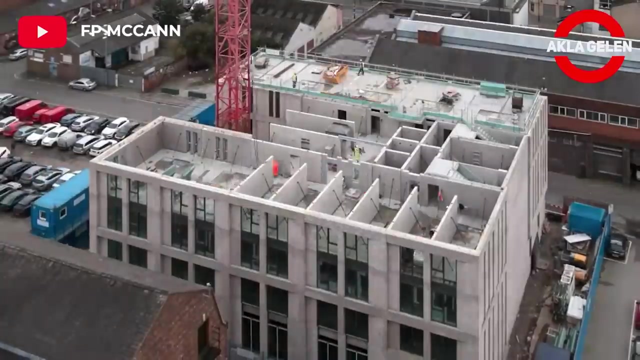 Precast construction can provide reduced time on site, reduced propping slash scaffolding costs, lower site labor costs and lower material storage costs With environmental impact. manufacturing in a controlled factory environment is more efficient than traditional construction, with less noise, air pollution and debris on site. 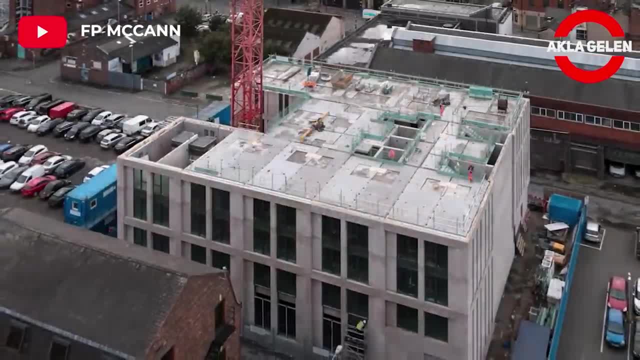 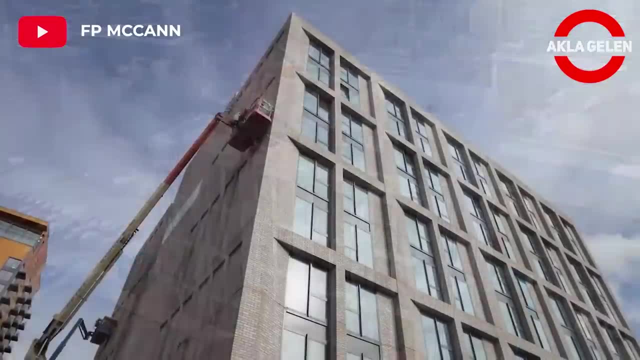 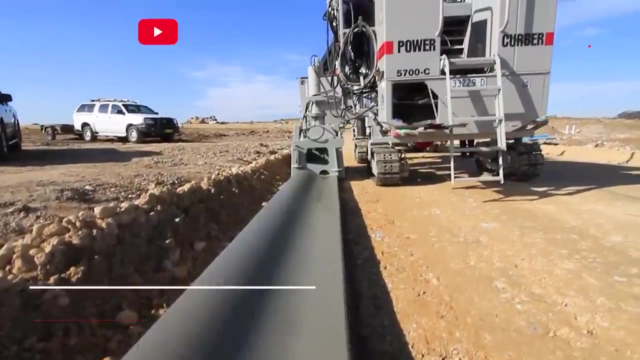 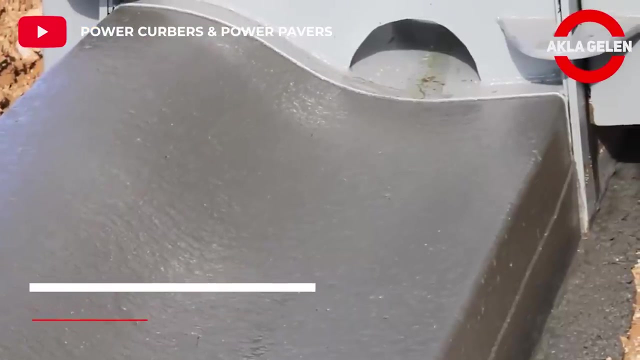 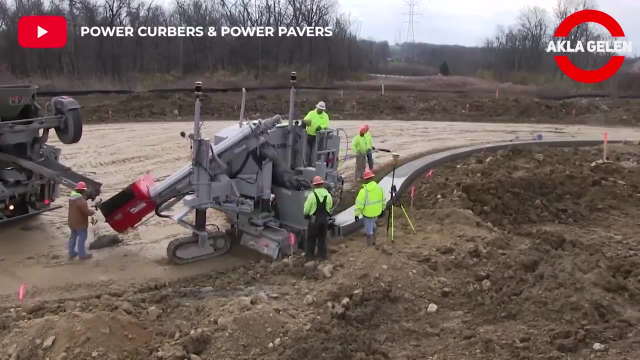 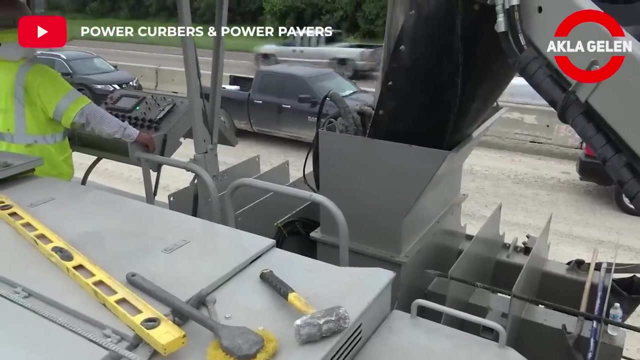 It uses recycled materials in production and allows benefits of thermal mass to be incorporated into designs. Slip Form Concrete Paving- The PowerKerber 5700C slip form paving machine pouring concrete curb using Topkin Millimeter GPS system. in Australia. The PowerKerber 7700 is a truly multipurpose machine designed for various offset and paving. 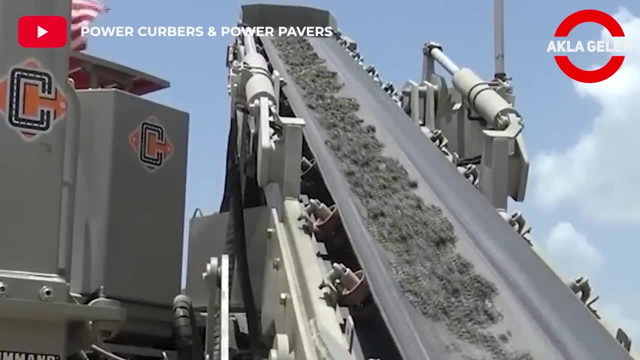 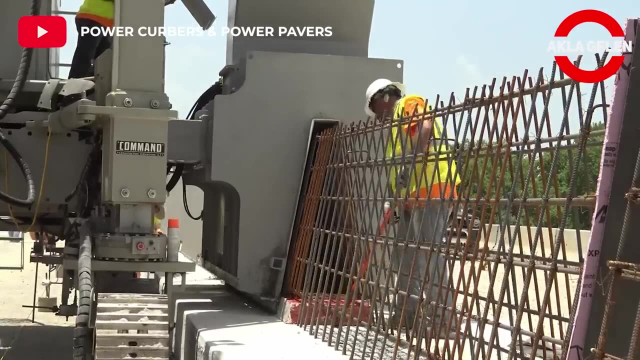 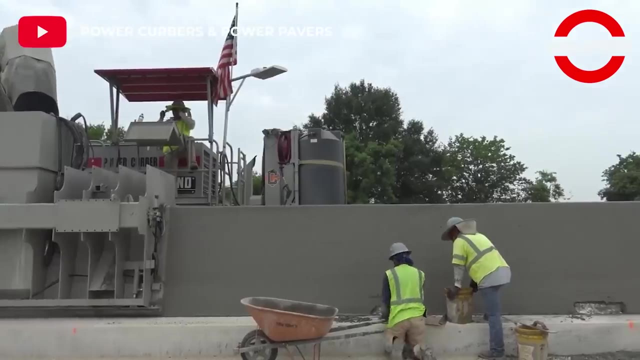 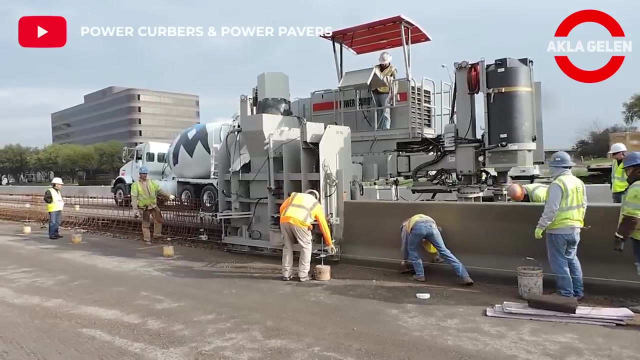 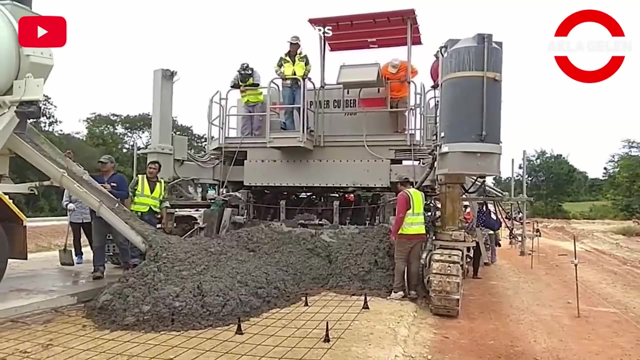 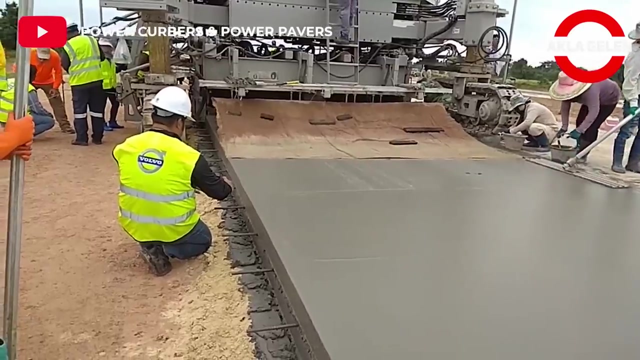 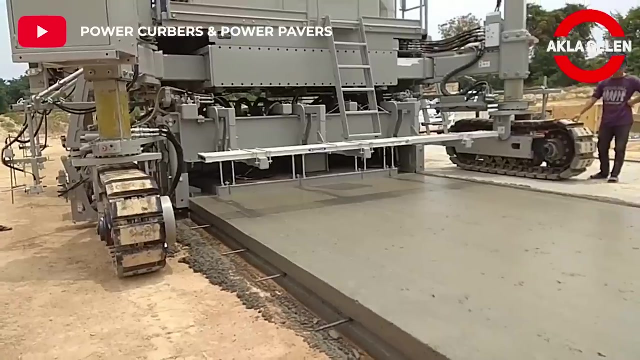 applications. We'll talk more about the technology that makes it possible to make a proactive contribution to part of yourма のerpa building sector within beast. This machine is used in highway barrier wall in road paving works. It is very enjoyable to watch the works done with this system. 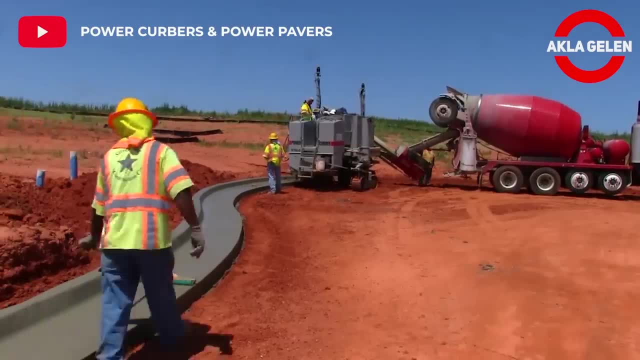 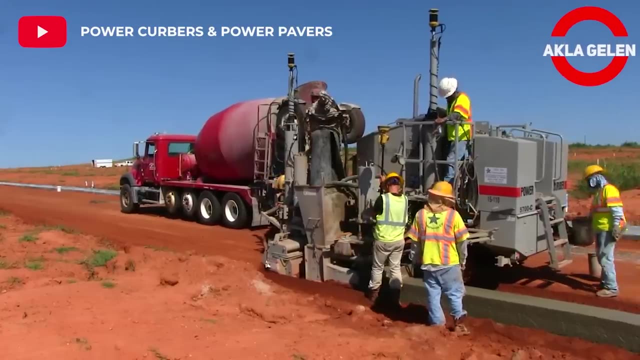 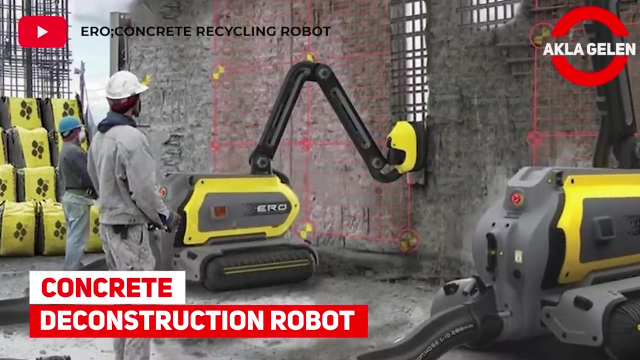 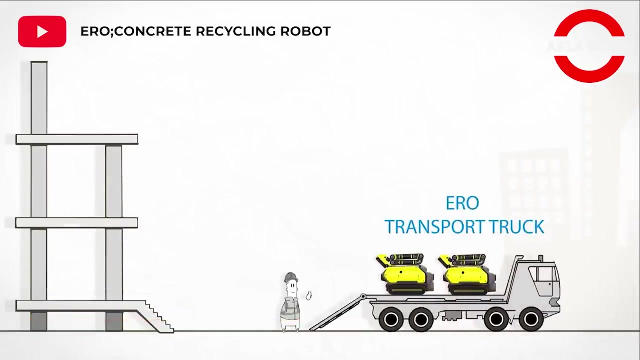 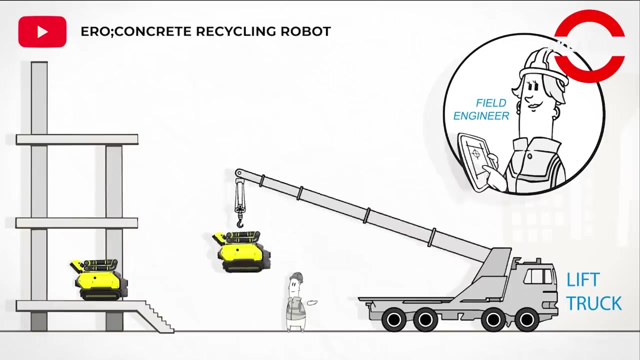 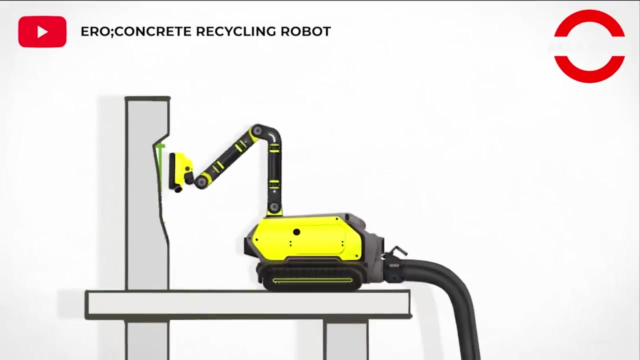 It's almost hypnotizing. Concrete Deconstruction Robot. ERO is a concrete deconstruction robot designed to disassemble concrete structures and enable the building materials to be easily disassembled. ERO uses water jets to crack the concrete surface to disassemble concrete and socks. 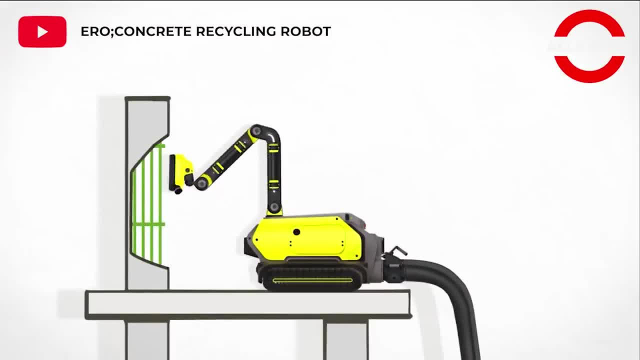 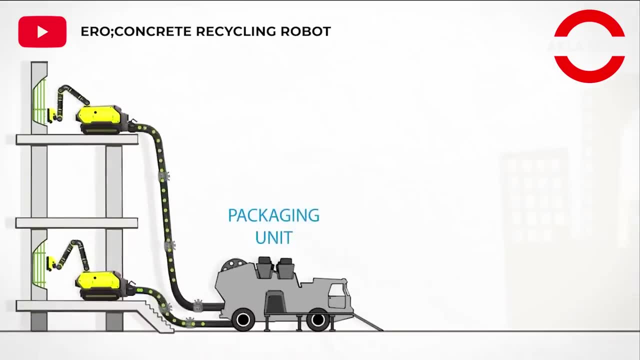 up the mixed debris. It cleanly separates the waste mixture and packages the clean material. What was previously waste now turns into labeled, packaged asset to be transferred right away into concrete pre-casting stations to be remolded into new building blocks. No dust, no waste, no separation. 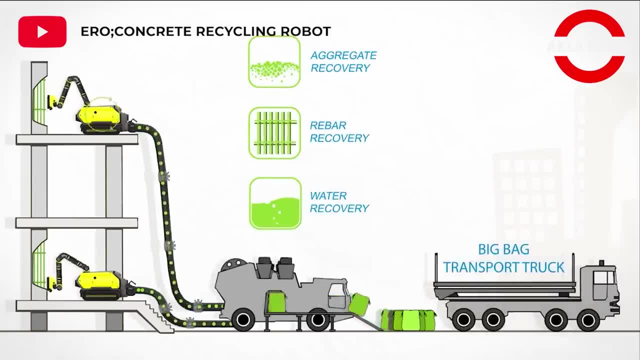 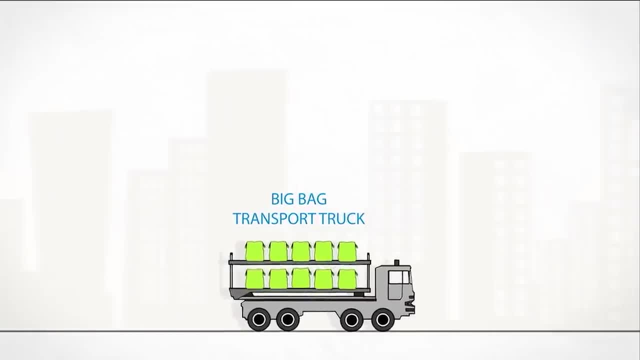 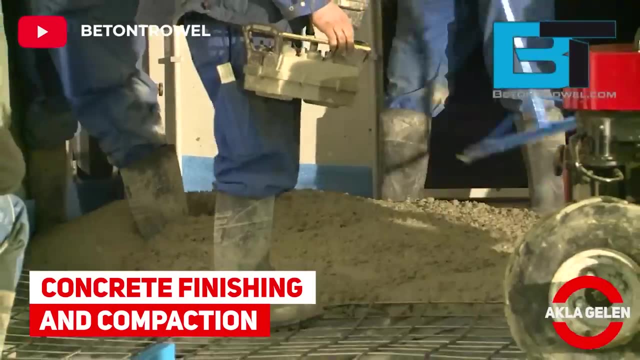 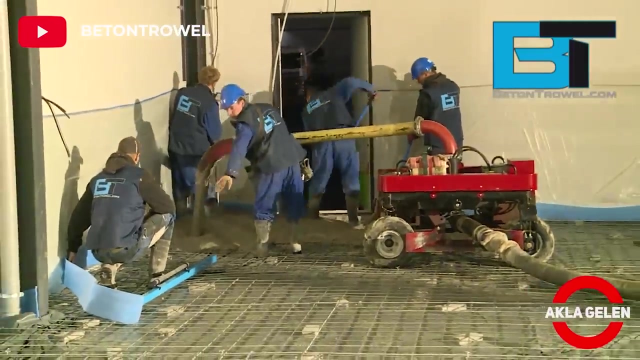 Only clean bags of aggregate and rust and dust-free rebar remains to be cut and reused directly. Concrete Finishing and Compaction. Comprehensive concrete finishing and compaction equipment makes work very easy. Concrete Finishing and Compaction. Concrete Finishing and Compaction. Concrete Finishing and Compaction. 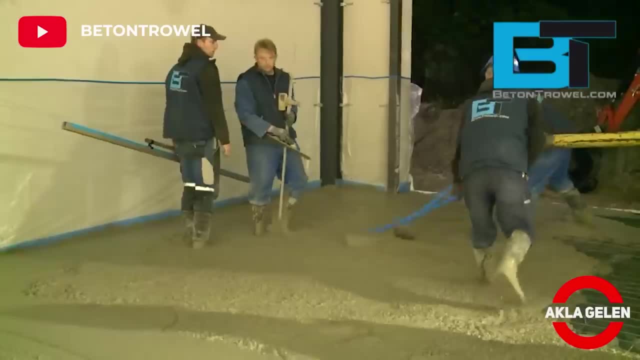 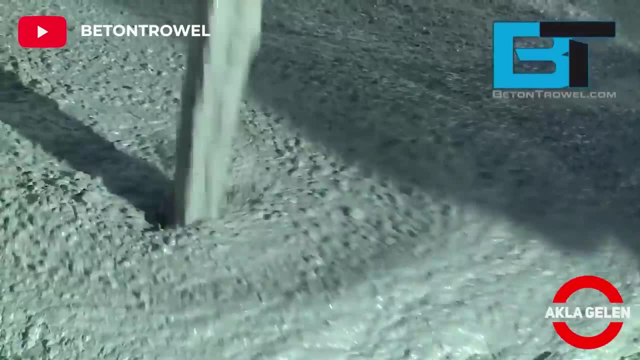 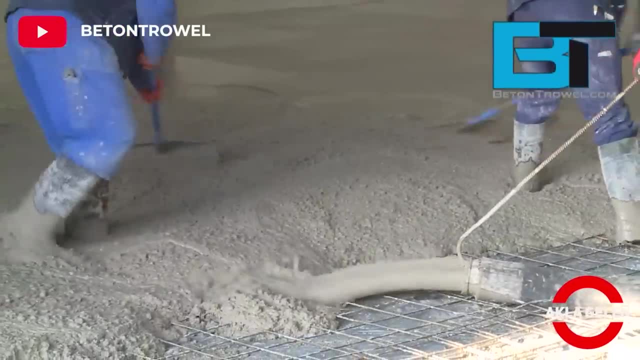 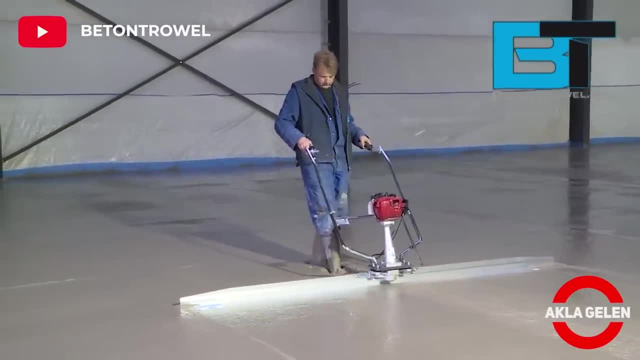 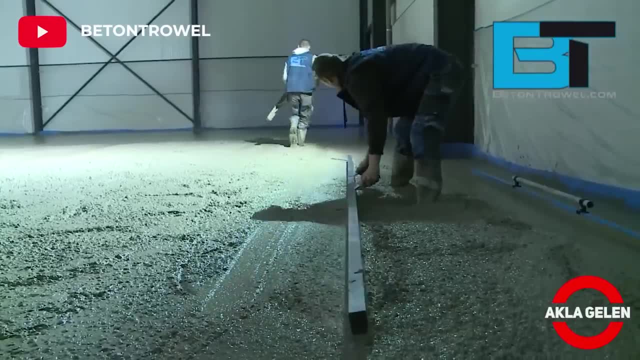 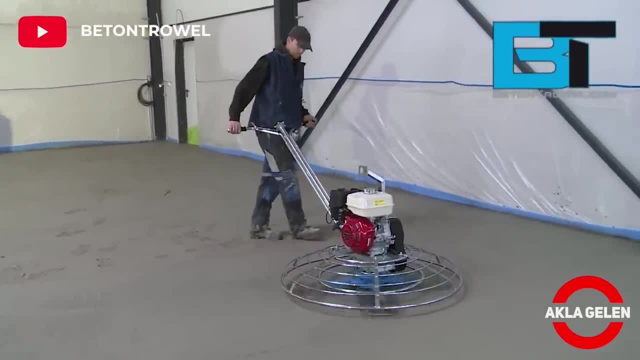 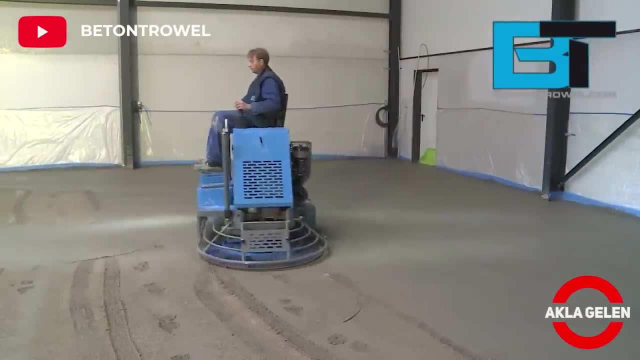